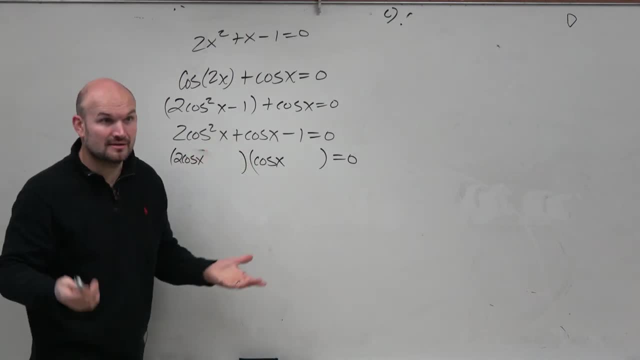 I mean, worst comes to worst, just guess right And say, oh, I made a mental error, right. But again, we can be a little smart about this. If 2 cosine of x, we want that to add, to be positive. 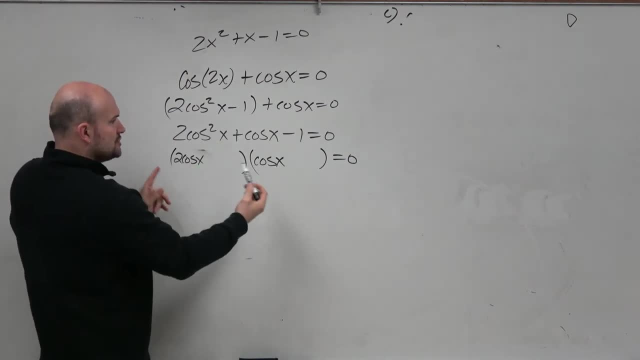 So, since the middle term is positive, we want the larger of our two products, our outer and our inner. those are the two products. We want the larger one of those to be positive, because you're going to combine terms, So that's why that's positive and that's negative. 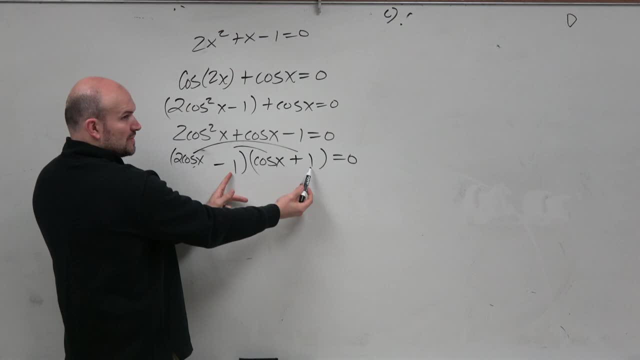 And again check my work: 2 cosine squared, multiply those that's negative: 1.. That's negative cosine of x. That's 2 cosine of x, 2 cosine of x, plus negative cosine of x. positive cosine of x. 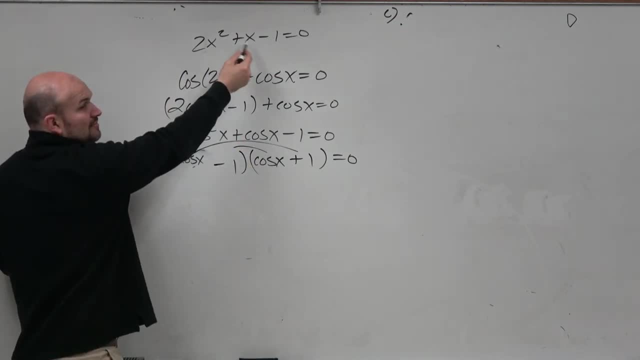 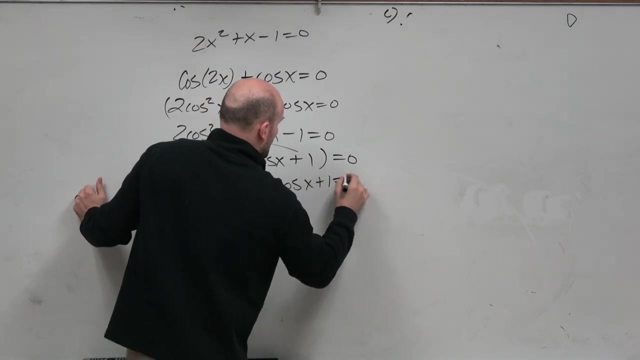 See how it works. And again, don't like that. Do the mental math with your x's. OK, But now, since I have a product equal to 0, I can apply the 0 product property. Man, so glad we did so much of that. 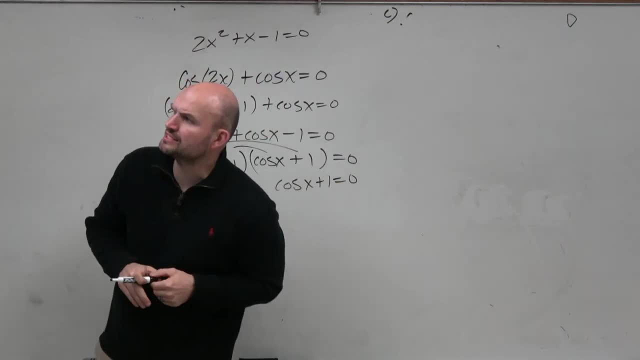 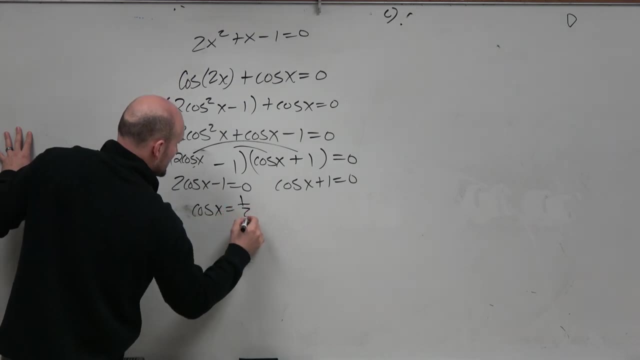 All right, then I can say: I think I asked you to find all the solutions on 0,, 2,, pi And all solutions. So let's do well, let's solve these first. So I use my inverse operations to isolate the trig function. 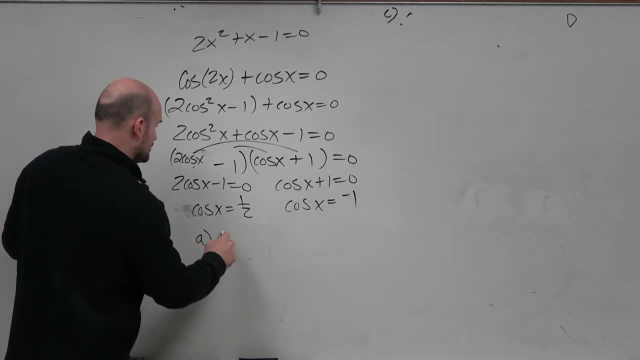 And then I can say: for all the solutions- I'm basically looking on the unit circle- When is cosine of x equal to 1 half? So cosine of x, let's see it's going to be pi over 3 and 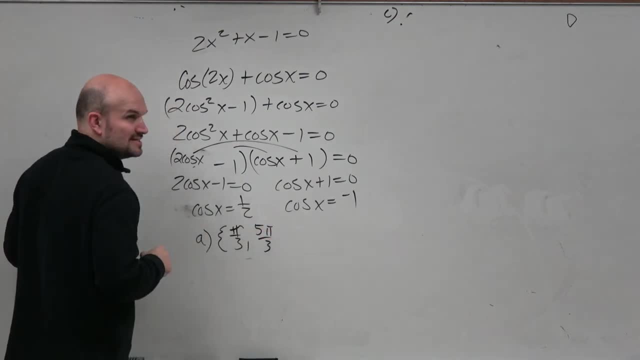 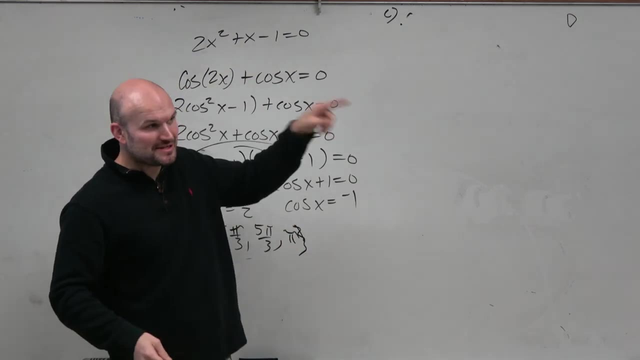 5 pi over 3, good. And then cosine is equal to the negative 1 hat 3 pi half Pi Right Negative 1 comma 0, so it's negative 1x. What did you say? 3 pi halves. 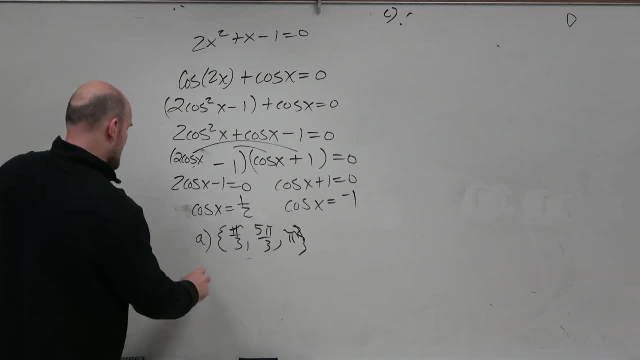 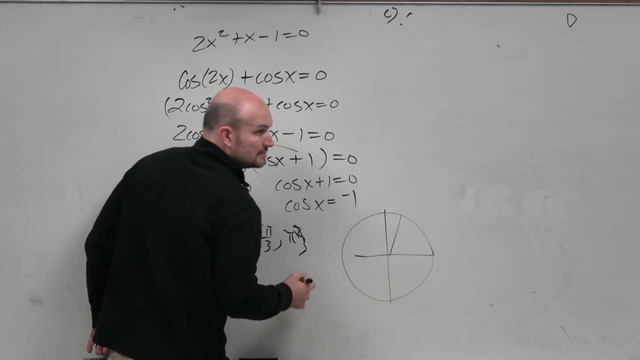 3 pi halves sine is equal to negative 1.. And then b, Now this one actually might be a thing. So what did you do? So we had sine, pi over 3,, 5, pi over 3, right, And again we knew it was those two angles, because they're. 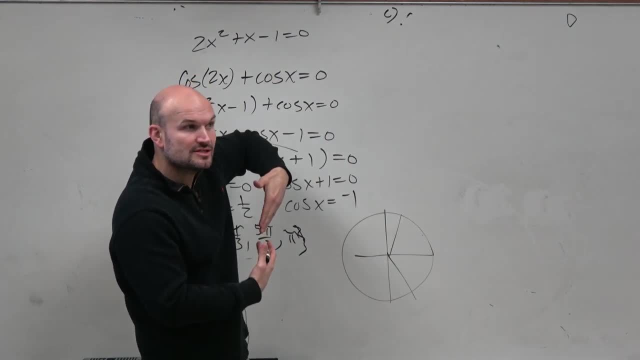 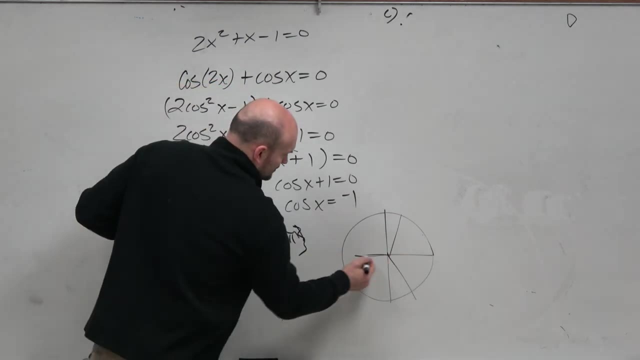 to the right of the y-axis right. If you had angles to the left, To the left of the y-axis, cosine would be negative Agreed. So that's why those two work. Now the last thing. then we have this angle.